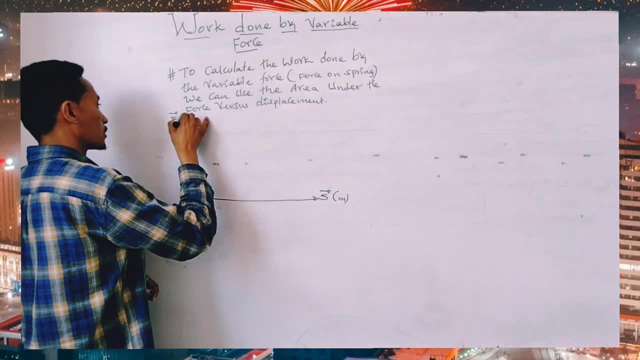 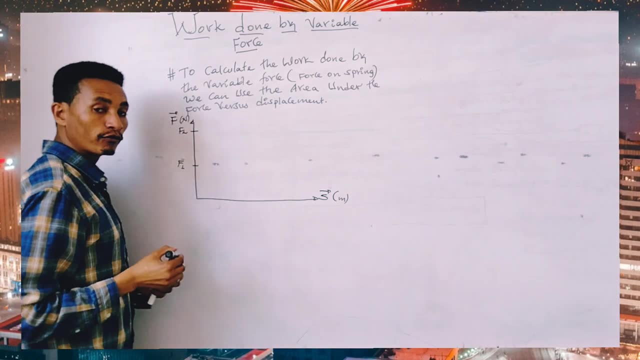 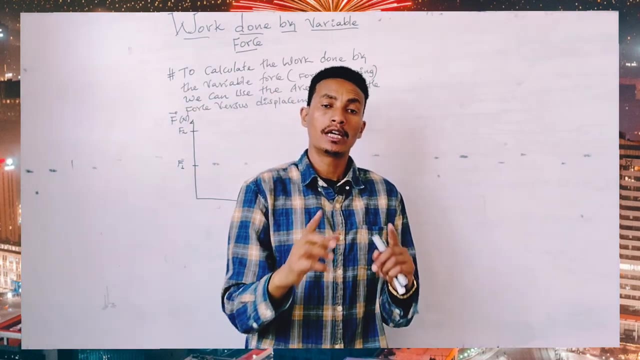 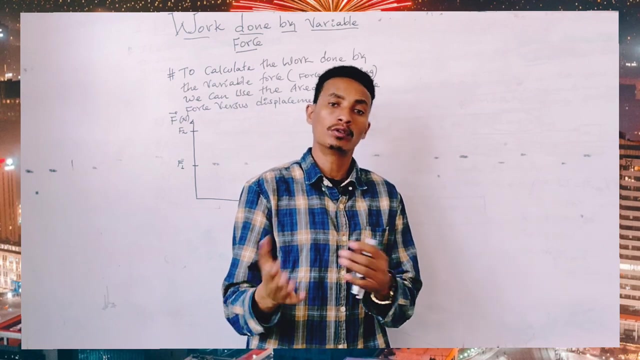 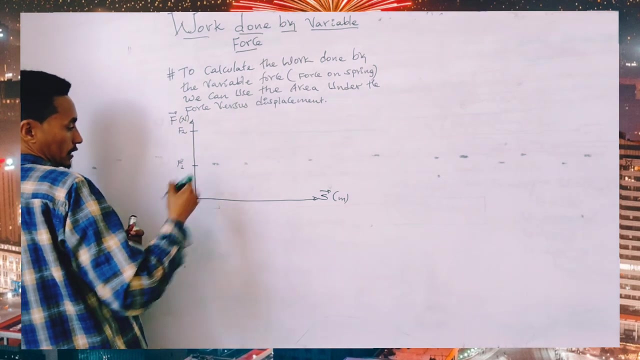 displacement, which is expressed by the unit of meter, Where this one is expressed in terms of Newton's. So here we have F1, F2.. This F1 and F2 are said to be variable force, But under system law, this is the area that we are going to calculate. So let's consider the system. 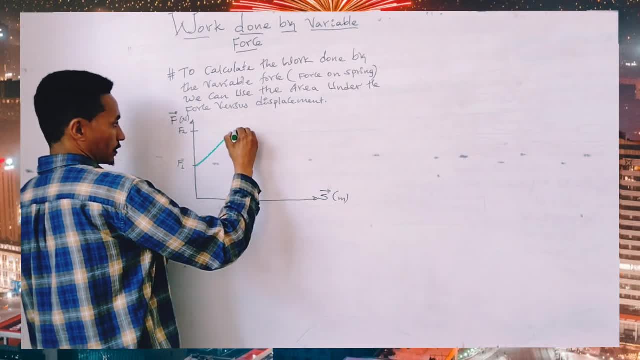 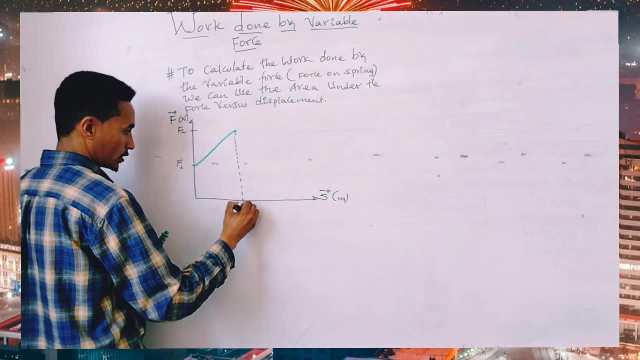 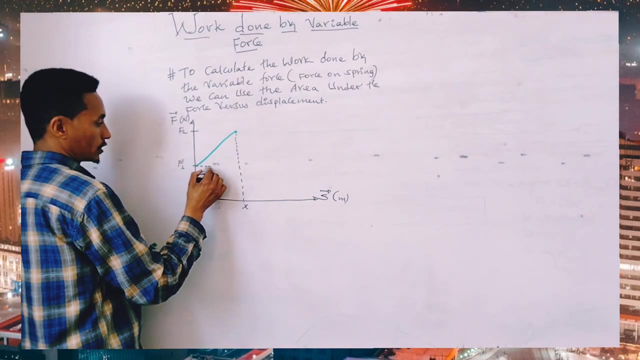 The variable system is expressed like this: So here let's express the system such Y, And let's say that here we have S1, or let's say the X. So here it is possible that these types of systems exist. So here we have an area. What types of area? 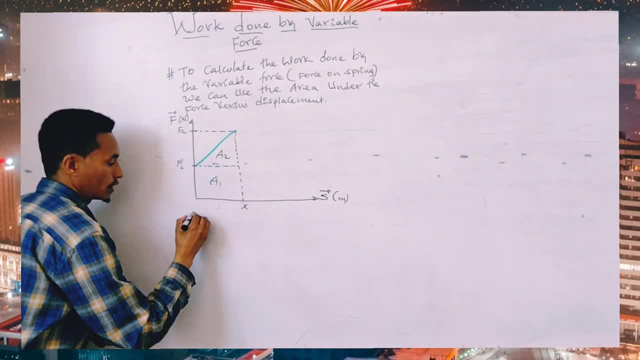 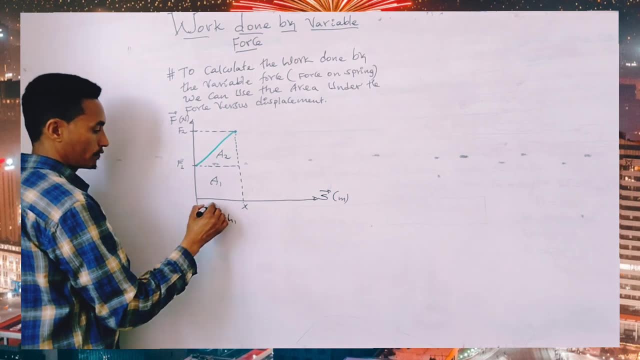 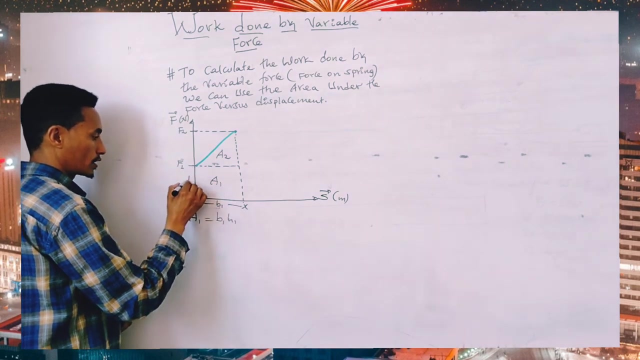 Oh yeah, A1. Here I have a 2.. So here it is possible that A1 is equal to B1 times H1. so here we have this: possible that, ah best, 1, which is equal to H1, S2, which is equal to H2.. 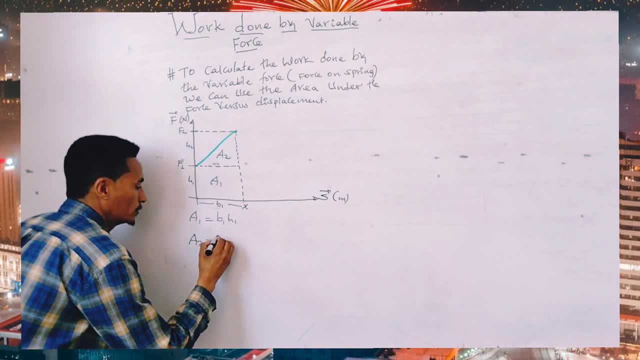 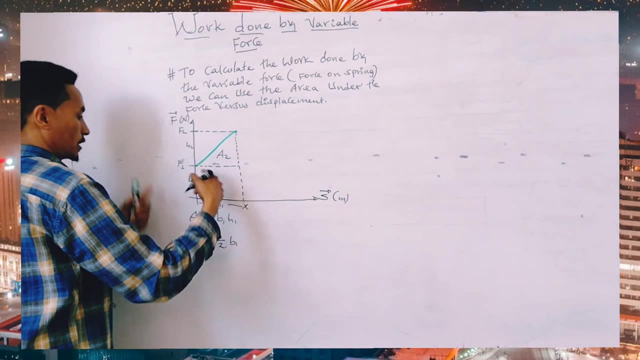 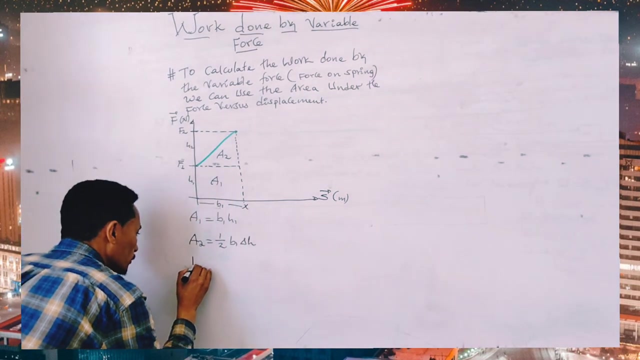 This is the first colon. Now we have the A2, and what is equal to A2? It seems like S1 over 2. times what their differences? so the difference is, it say, to be that change of what change of? so, finally, the work done by the variable force it is equal to. it seems like a1 plus a2. 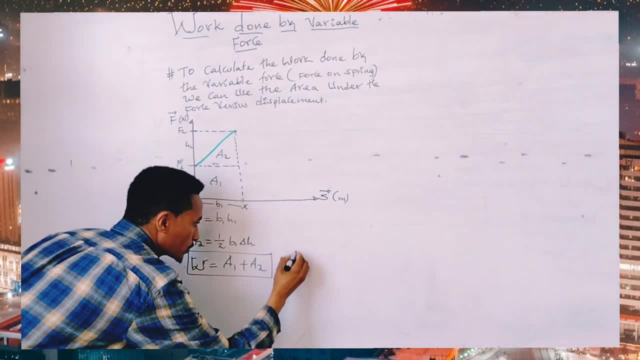 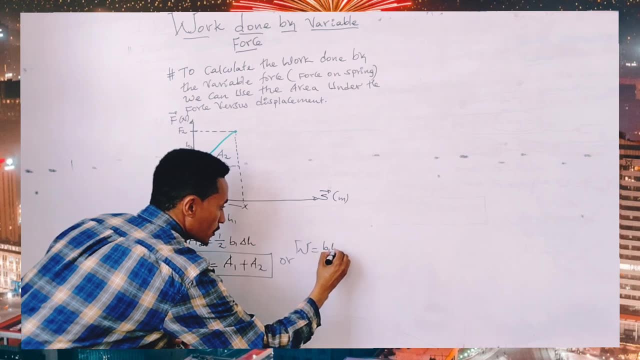 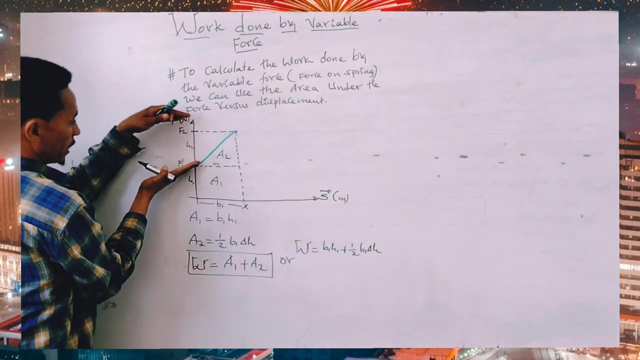 or it is possible that the work done by the variable force is equal to, for say types of system, it's possible that b1, h1 plus 1 over 2 b1 times a change of h. this is the way how we're going to just equate the work done by variable force. 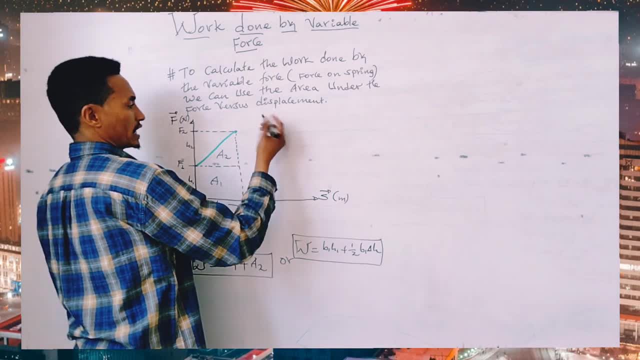 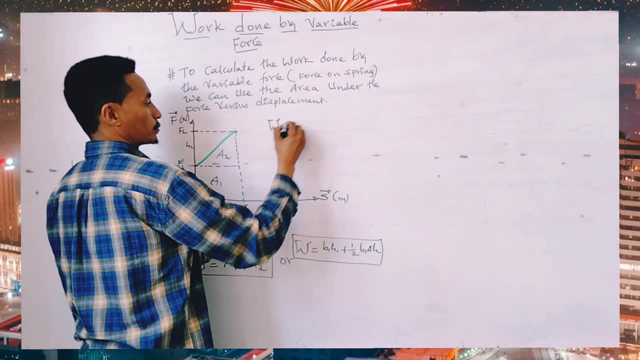 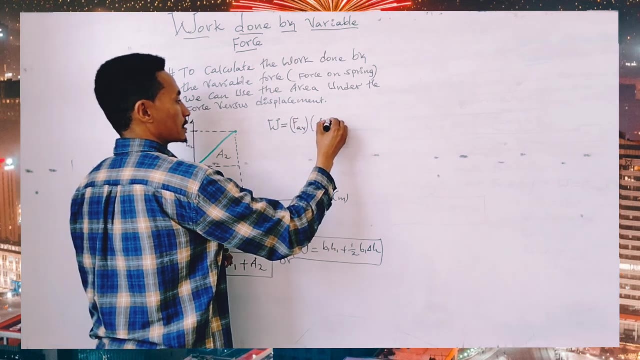 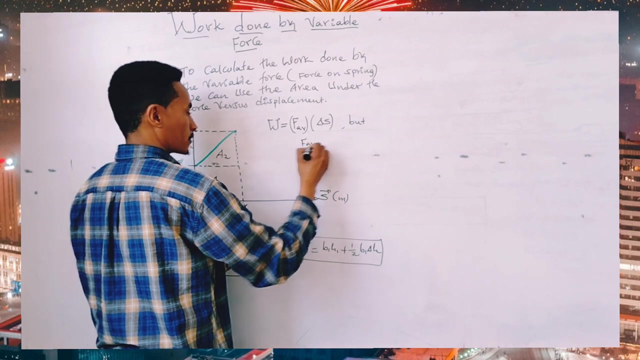 or easily by the expression. it's possible that the work done by the variable force it is equal to. it is possible that the force, what types of volt? the average force times the change in distances, the change in distances. but it is possible that the average force- here we have f1 and f2.